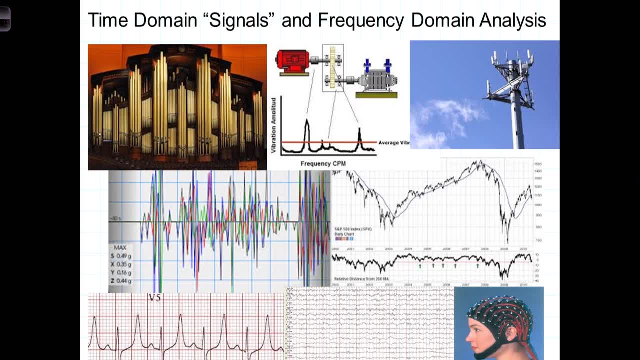 Many time domain, events and signals lend themselves to analysis and understanding in the frequency domain, For example, music. When we listen to music, we appreciate the low tones and the high tones, which all exist concurrently in time, Yet to fully understand them or to 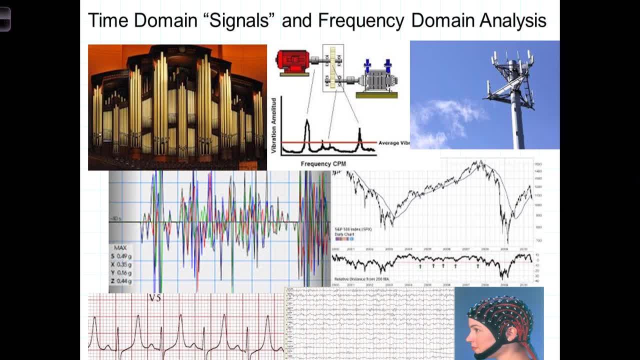 speak about what's taking place in the music. we do talk about low tones or tones that are oscillating at lower frequencies, higher pitches which are oscillating at higher frequencies. Vibrational analysis of a mechanical system lends itself to frequency domain analysis. 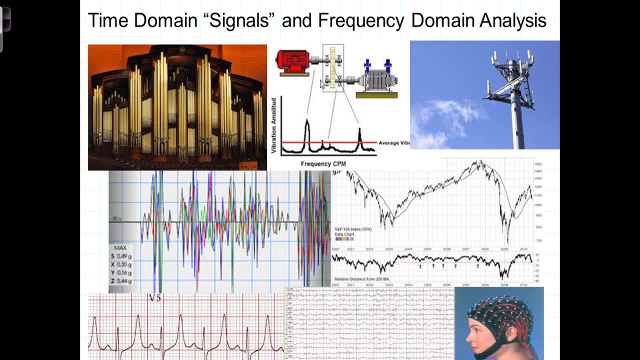 where vibrations or frequencies introduced by different parts of the system can be identified in the frequency domain. Broadcast radio and cell phones are all defined in terms of the frequency domain. We talk of the frequency of a radio station: 88.3 megahertz or one. 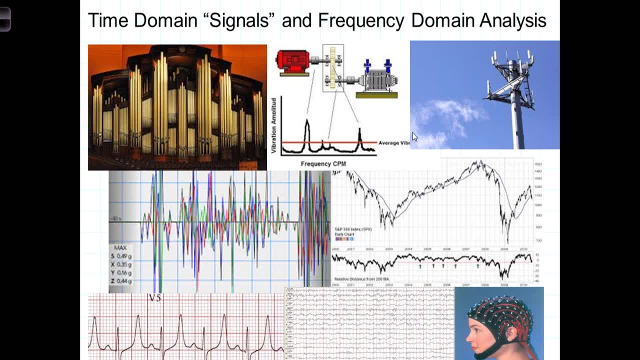 oh three point five megahertz. As we'll see, the frequency spectrum, the electromagnetic spectrum, is divided up into channels of frequencies. Seismic activity lends itself to frequency domain analysis. Analyzing the lower, slower traveling compression waves and then more rapidly propagating higher frequency waves allows understanding of what's taking place. 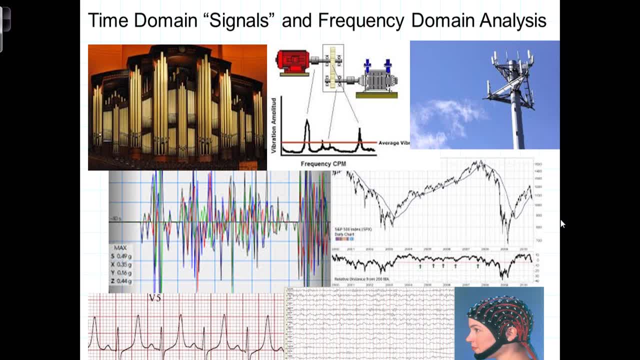